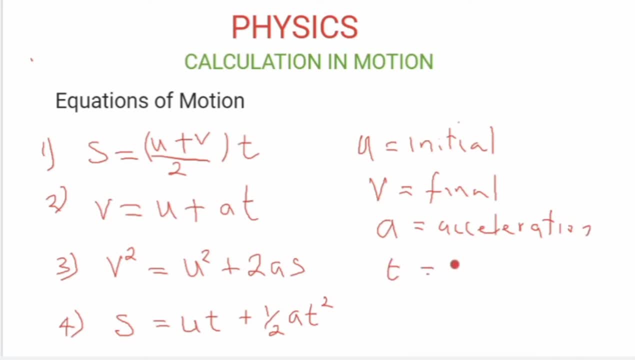 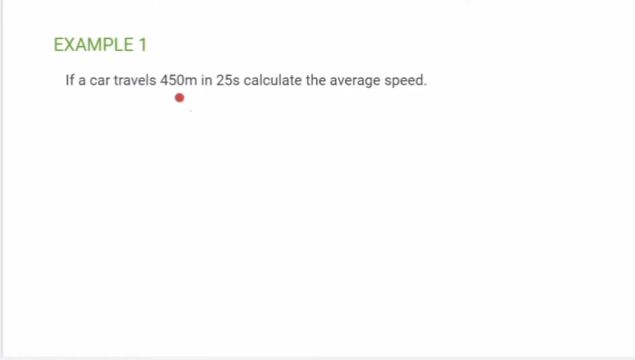 T represent time and you will see T in the equation means time. then, finally, X represent distance. okay, present distance. so let's begin the calculation. example one: if a car travels 450 meter in 25 seconds, calculate the average speed. remember the average speed is the speed of the car. 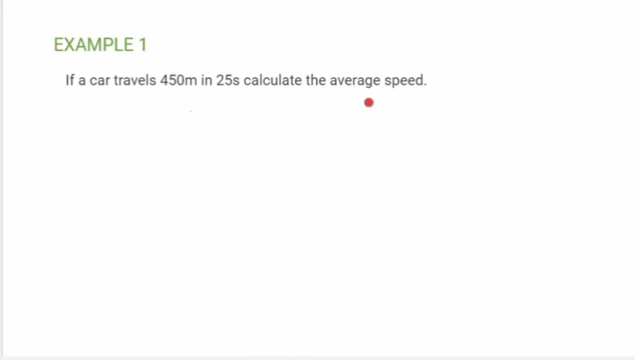 remember: average speed is total distance divided by total time. first we're going to state our parameters. solution S is given to us as 450 meters. okay, T, which is the total time, is given to us as 25 seconds. so to get the average speed, we'll be equals to the total distance S over the time. so just do substitution. 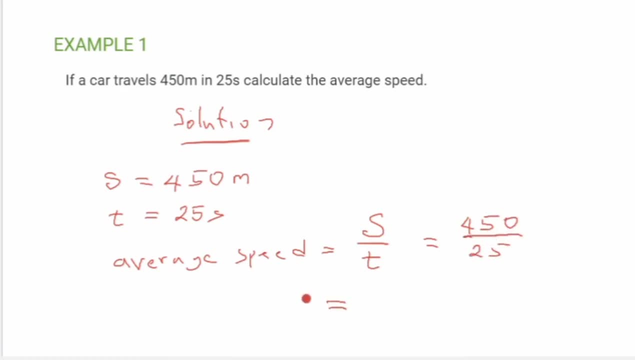 divided by 25, that gives us the average speed as 18 meters per second. so average speed V equals 18 meters per second. let's go to the next question. example two: a train starts from rest and travels with a uniform acceleration of 0.5 meters per second square for 20 seconds. calculate its final Velocity and distance covered. 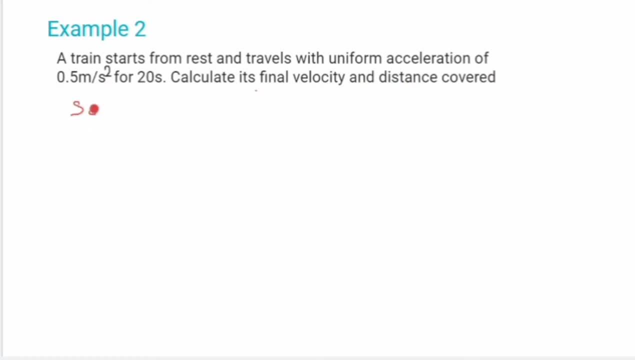 we're looking for final Velocity and the distance covered, so first we'll write. our solution will bring out our parameters. a train starts from rest, body starts from rest. in physics it means that the initial velocity is equals to zero. okay, if your body starts from rest, initial velocity is equals to zero, all right, we are given acceleration. 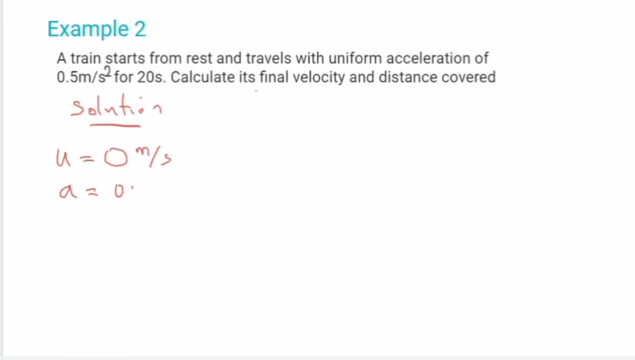 a as 0.5 meters per second square. they were given time, t as a 20 second, and then we are to find the final velocity, v, okay, and then the distance covered, s. so that's what we are looking for: to know the equation to use to solve. 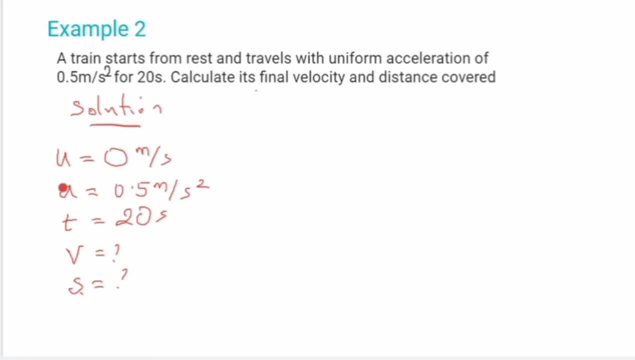 this equation. we are going to use the equation to solve this equation problem. we look at the equations of motion that have u, a, t and v, so we can find the value of v. so check the equations which of the equation have u a, t and v, so we can substitute these values. 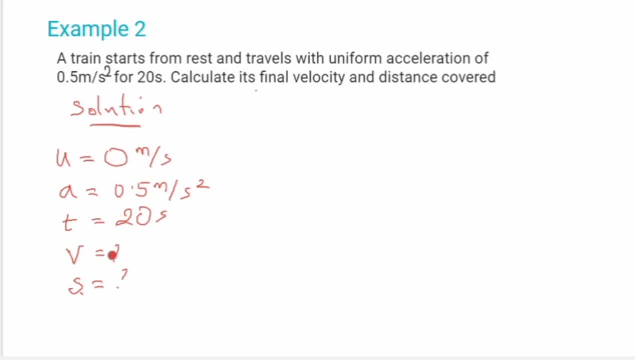 that we know and find the value we don't know. so if you check the equation critically, the equation that have the four parameters is the second one v. the equation that have the four parameters is the second one v. the equation that have the four parameters is the second one. v. equals u plus a t. okay, so i can find my v. 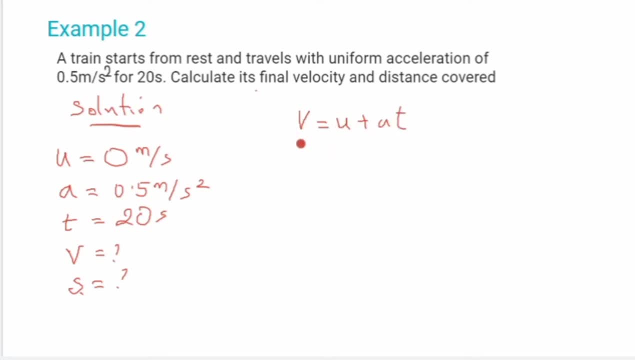 equals u plus a t. okay, so i can find my v. equals u plus a t. okay, so i can find my v. i know u, i know a and i know t, so substituting my value v. i know u, i know a and i know t, so substituting my value v. 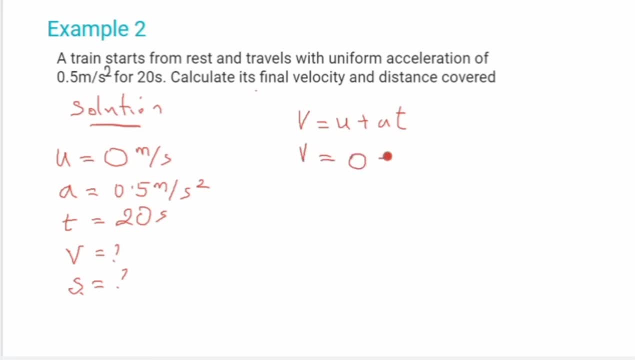 i know u, i know a and i know t, so substituting my value, v will be equals to u, which is 0. will be equals to u, which is 0. will be equals to u, which is 0, plus a, which is 0.5. 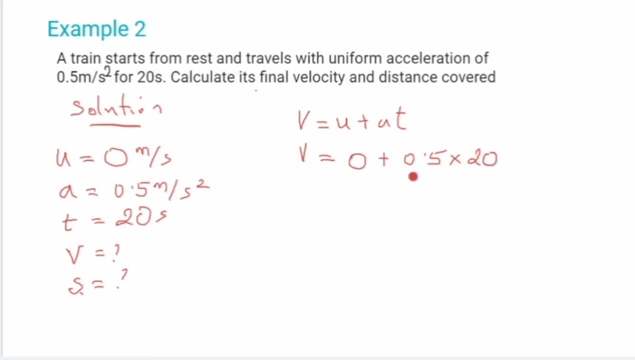 plus a, which is 0.5. plus a, which is 0.5. okay, times t, which is 20. okay, times t, which is 20. okay, times t, which is 20. okay, so v is equals to zero. okay, so v is equals to zero. 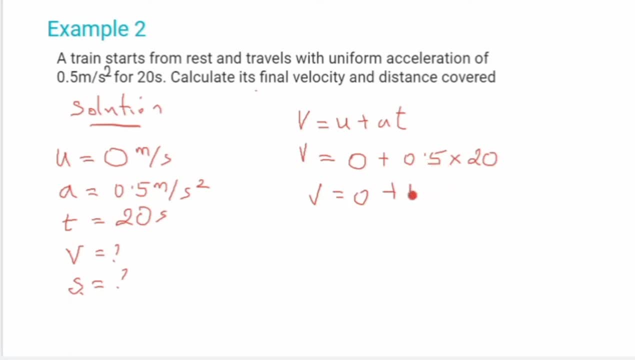 okay, so v is equals to zero. plus 0.5 times 20 will give us 10, so v will now be 10 meters per second. is that okay? now to find our distance, we can use any of the equations that have distance, any of them, so let's use the first. 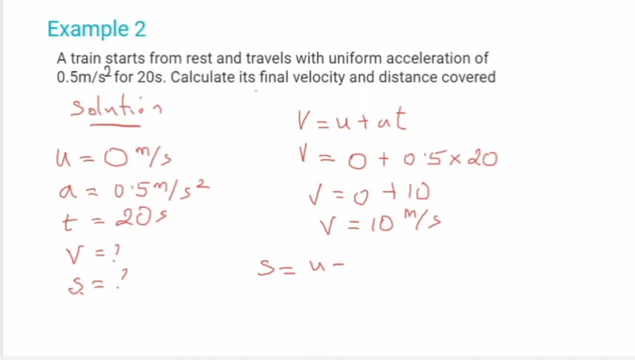 one s equals u plus v over 2 right times time. so u is 0 plus v, which is 10 divided by 2, then times the time 20.. okay, so that will give us 0 plus 10 is 10, 10 divided by 2. 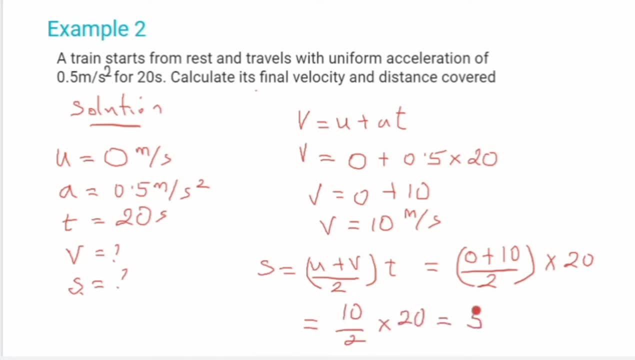 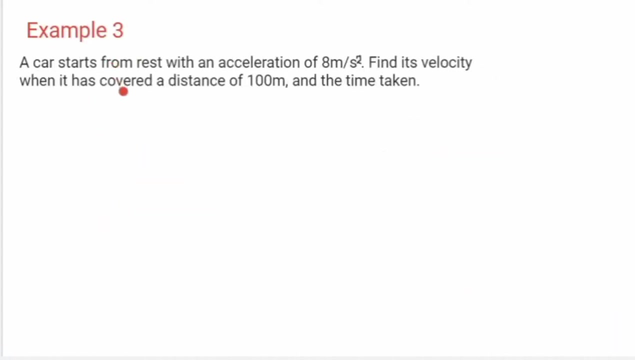 times 20.. 10 divided by 2 is 5 times 20, so we are going to have 100 meters. that's our answer. so any of the equation you use that have distance, you'll be able to get the same answer. example 3: now a car starts from rest with an acceleration of 8 meters per second square. 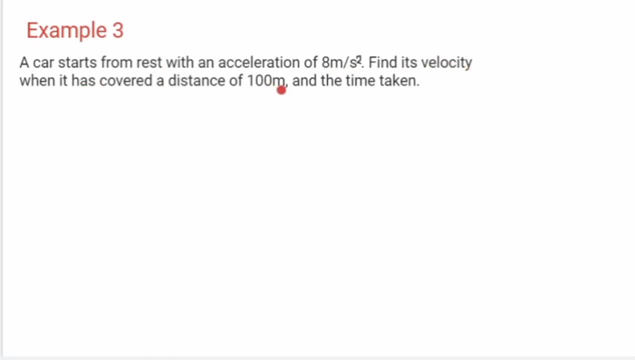 find its velocity when it has covered a distance of 100 meter and the time taken: okay. so solution: the parameters: first start from rest. u is equal to 0 meters per second. okay. the acceleration: a is equals to 8 meters per second square. the distance covered: s is equals to. 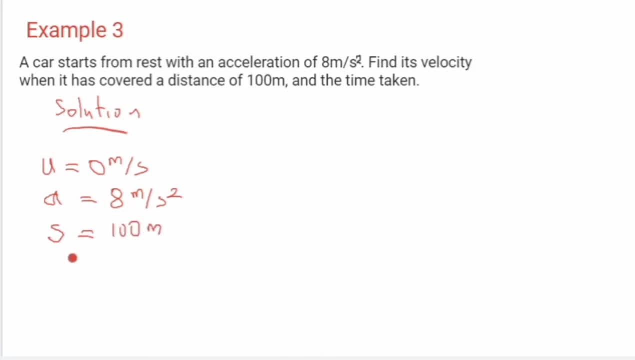 100 meters, and then we are looking for the velocity. that's the final velocity. we are also looking for the time taking. so which of the equation are we using? we have u, we have a, we have s and we need to look for v first. but if you check the equation of motion, we're going to. 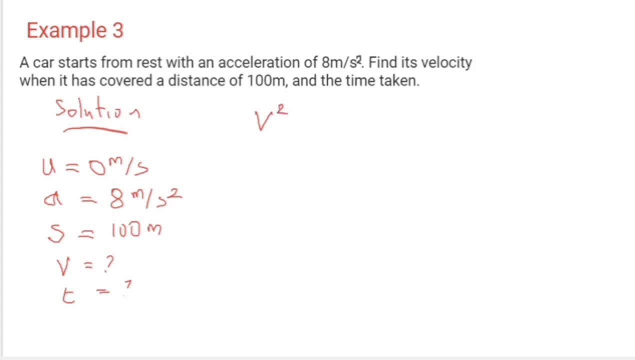 be using: v square equals u square plus 2 a s. all right to find v first. so v squared equals u, which is zero, squared plus 2 times a, which is 8, then times s, which is 100. so v squared equals to 0 squared, which is 0 plus 2 times. 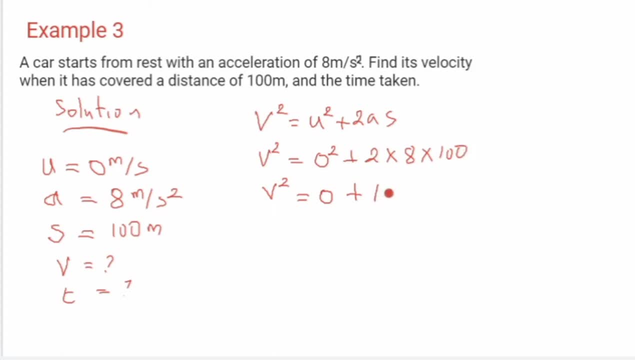 8 is 16 times, this will give us 1, 2 times 8 16 times. this will give us 1, 2 times 8 16 times. this will give us 1 six zero zero. all right, okay, so v square will not be equals to one six zero zero, so it means: 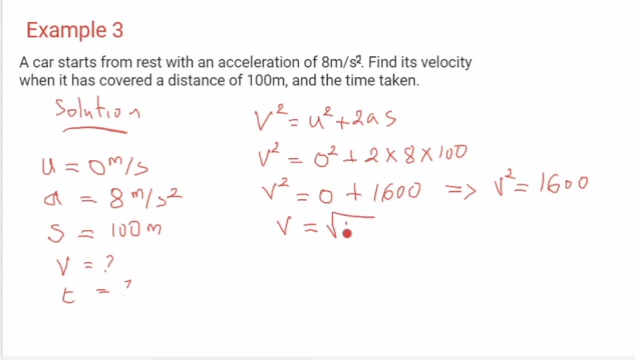 we find the square root of one six, zero, zero also will be 40 meters per second. is that okay, 40 meters per second? all right. to find the time taken, we can use any of the equation of motion, the half time. so if we use v equals u plus a, t, we can find this t. 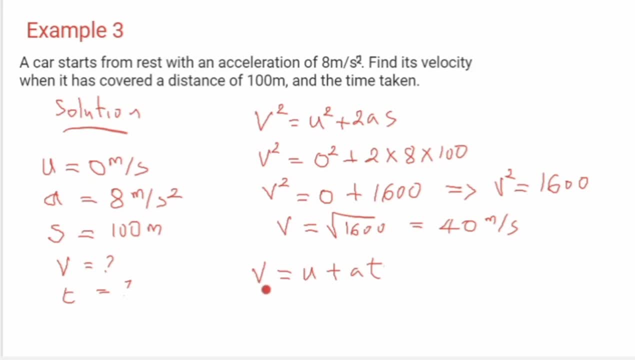 okay, v is 40. so 40 equals u, which is zero, plus a, which is eight t. okay, zero plus this, this is zero. so meaning that 40 will be equals to 8 t. divide both sides by 8, we're going to have 40 over 8 equals 8, t over 8. 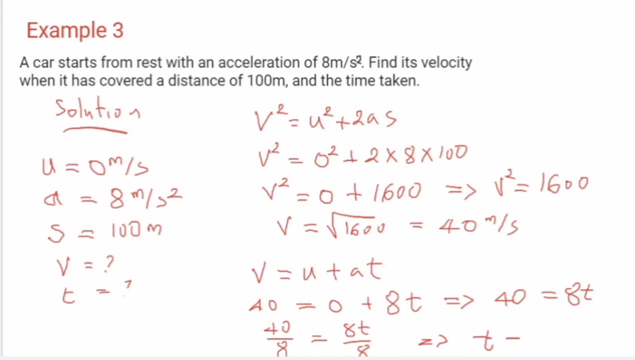 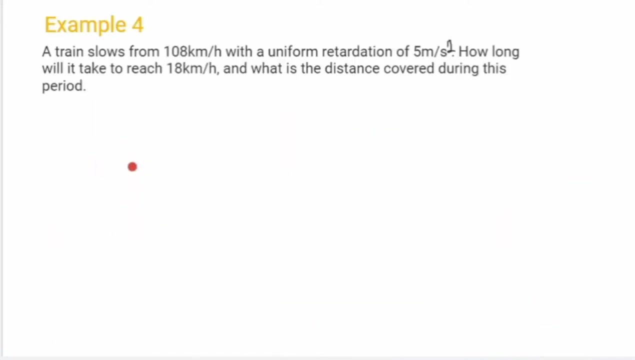 all right. so therefore t will now be equals to 40 over it, which is 5 seconds. that becomes our answer. all right, one more question: train slows from 1, 0, 8 kilometer per hour, with the uniform retardation of 5 meters per second square. how long will it take to reach 18 kilometer per hour? and 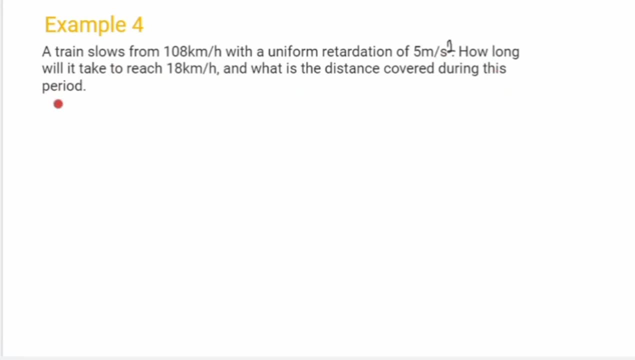 what is the distance during this period? all right, so solution slows from this velocity. so that's my initial velocity: 108 kilometer per hour. we need to convert it to meters per second. so to convert it to meters per second multiplied by 1000, divided by 60 times 60, all right, this will give us 30. 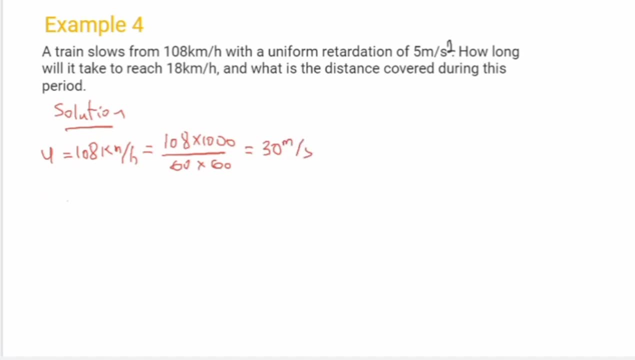 meters per second. retardation is negative acceleration, so a equals minus five meters per second square. okay. and then the final velocity is given to us as V: 18 kilometer per hour. to convert it multiplied by 1000, divided by 60 times 60: okay, that will give us five meters per second, okay. so we are looking for the. 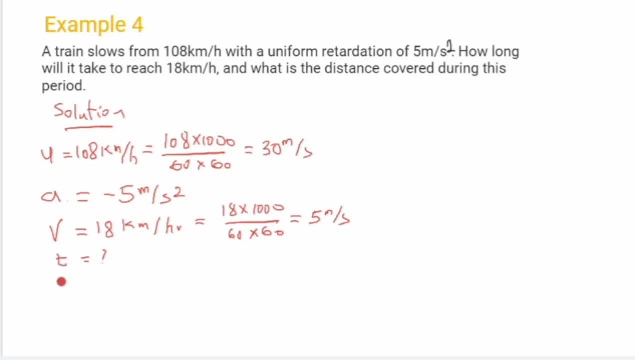 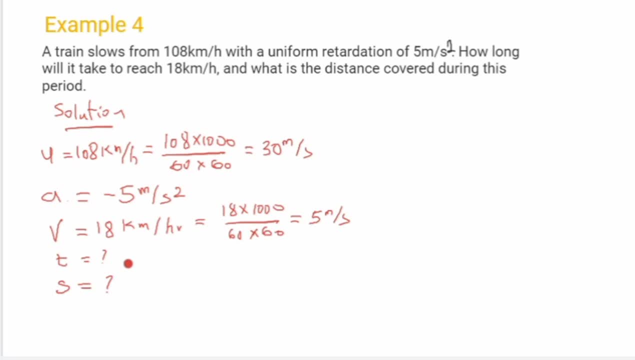 the distance cover. so, to get the time, which of the equation are we going to use? of the equation are we going to use? of the equation are we going to use? we're going to use though we have you. we're going to use though we have you. 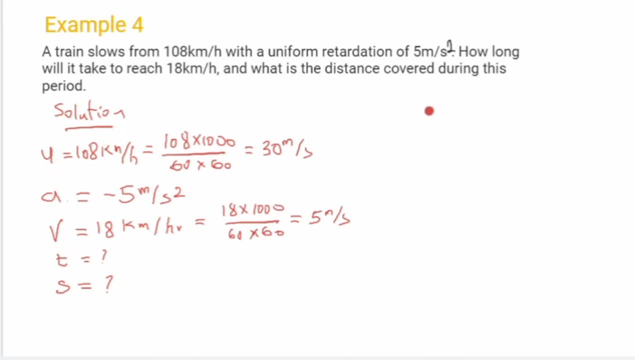 we're going to use- though we have you, we have a, we have V and we have T- we're we have a, we have V and we have T, we're we have a, we have V and we have T. we're going to use: V equals u plus 80 to get. 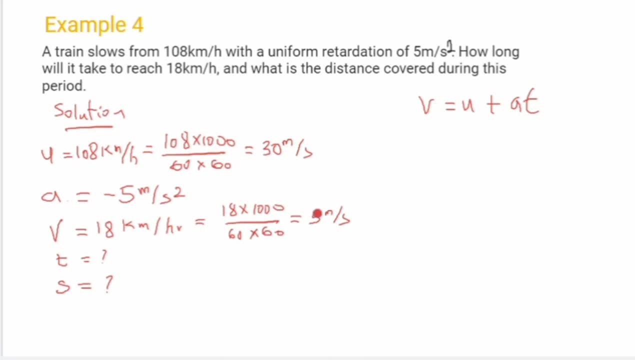 going to use V equals u plus 80 to get. going to use V equals u plus 80 to get our time. so V is 5: 5 equals u is 30, our time. so V is 5: 5 equals u is 30, our time. so V is 5: 5 equals u is 30 plus a is negative 5 times T that we're. 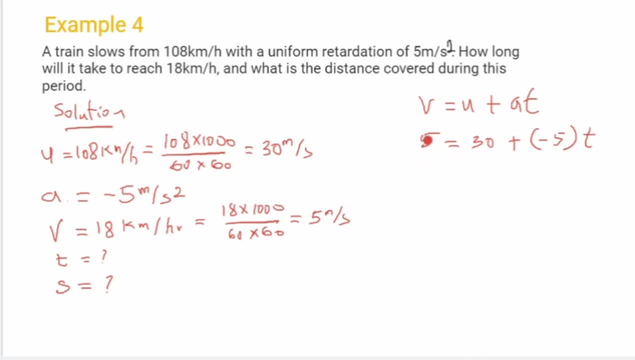 plus a is negative 5 times T that we're plus a is negative 5 times T that we're looking for. okay, move this 30 to this looking for. okay, move this 30 to this looking for. okay, move this 30 to this side. so 5 minus 30 equals to minus 5 T. 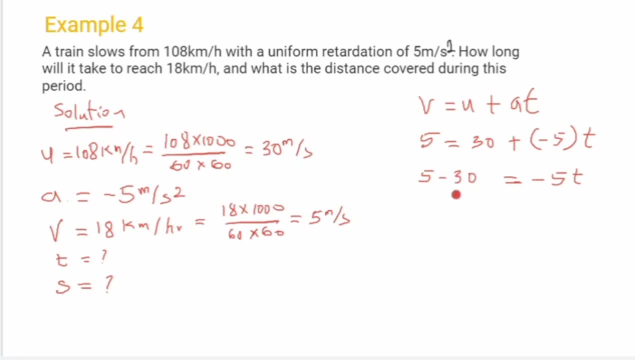 side, so 5 minus 30 equals to minus 5 T side, so 5 minus 30 equals to minus 5 T. okay, okay, okay. 5 minus 30 will give us minus 25. 5 minus 30 will give us minus 25. 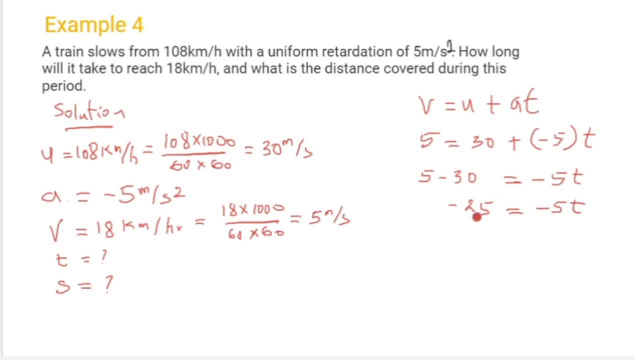 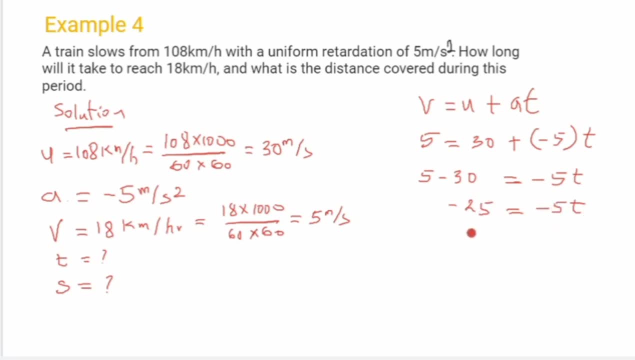 so divide through by 5. you divide the hour minus 5. we have T divided our minus minus 5. we have T divided our minus minus 5. we have T divided our minus 5. we're going to have T as 5 seconds. 5. we're going to have T as 5 seconds. 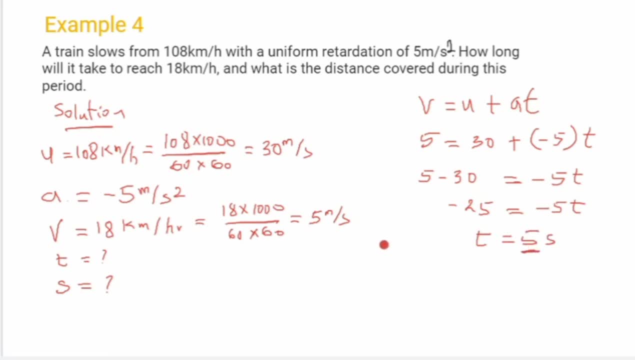 5. we're going to have T as 5 seconds. that's our answer. but to find the, that's our answer. but to find the, that's our answer. but to find the distance, you use any of the equation distance. you use any of the equation distance. you use any of the equation that have distance, you can use equation. 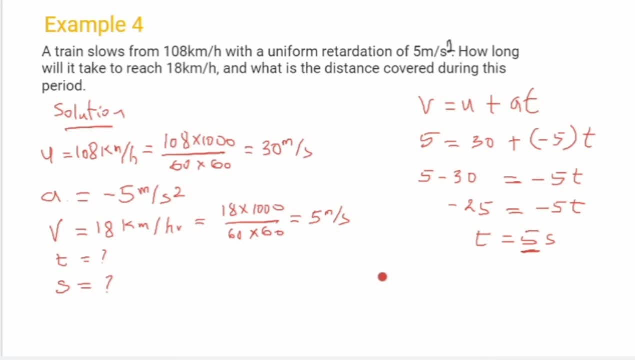 that have distance. you can use equation that have distance. you can use equation 1 or equation 3 or equation for any of 1 or equation 3 or equation for any of 1 or equation 3 or equation for any of them, so we can decide to use them. 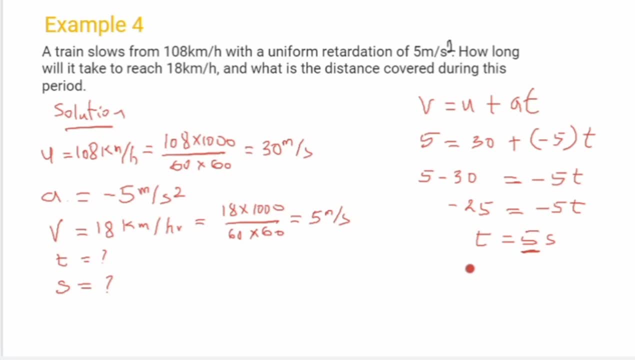 them, so we can decide to use them. them, so we can decide to use them. anyone V square cos u square plus 2 s, or anyone V square cos u square plus 2 s, or anyone V square cos u square plus 2 s, or we use just a simple one: s equals u plus. 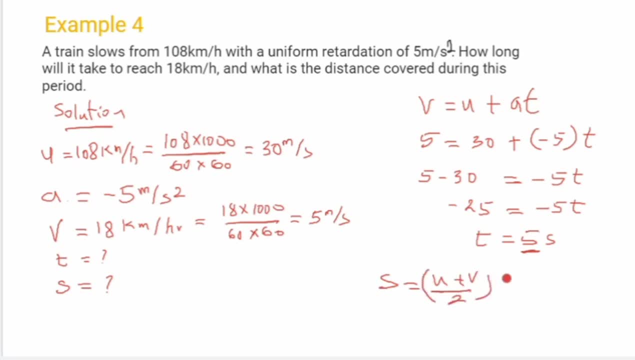 we use just a simple one: s equals u plus. we use just a simple one: s equals u plus V. over 2 times time. we're still going to V over 2 times time. we're still going to V over 2 times time. we're still going to get our answer: okay, you is 30 plus V is. 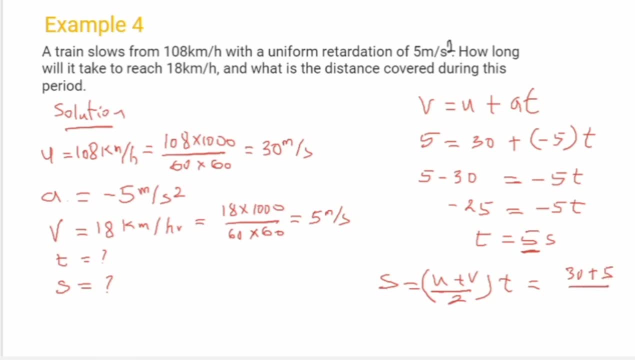 get our answer: okay, you is 30 plus V is. get our answer: okay, you is 30 plus V is 5- 5, 5 over 2, and then times T, which is 5 okay over 2, and then times T, which is 5 okay. 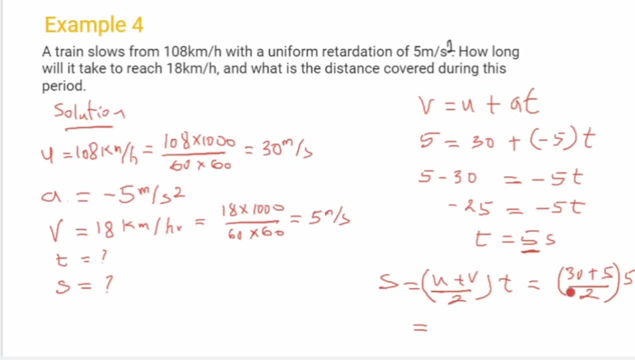 over 2, and then times T, which is 5, okay. so 30 plus 5 will give us 35 over 2. so 30 plus 5 will give us 35 over 2. so 30 plus 5 will give us 35 over 2 times 5. okay. so when you multiply 35, 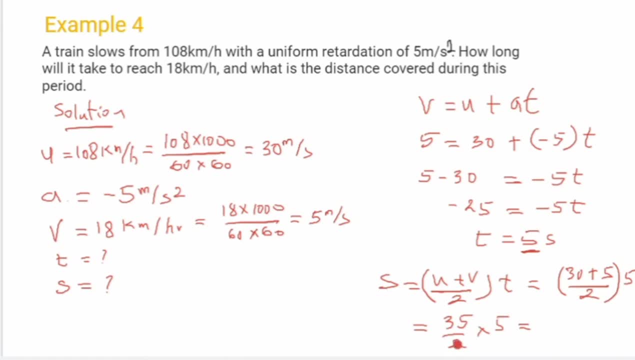 times 5: okay. so when you multiply 35 times 5, okay. so when you multiply 35 times 5 divided by 2, you are going to times 5 divided by 2, you are going to times 5 divided by 2, you are going to get 80- 7.5. that's our answers in meters. 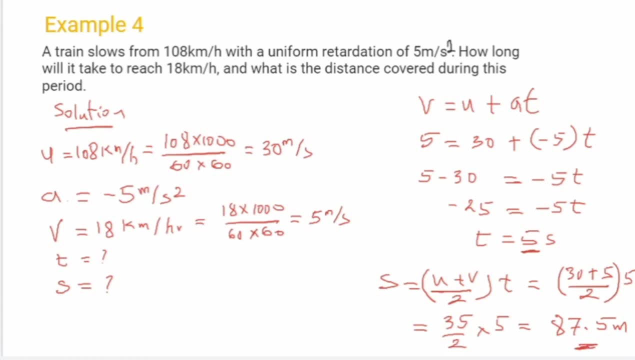 get 80- 7.5. that's our answers in meters. get 80- 7.5. that's our answers in meters. don't forget to put your units right. don't forget to put your units right. don't forget to put your units right. that becomes our answer. it is 7.5 all. 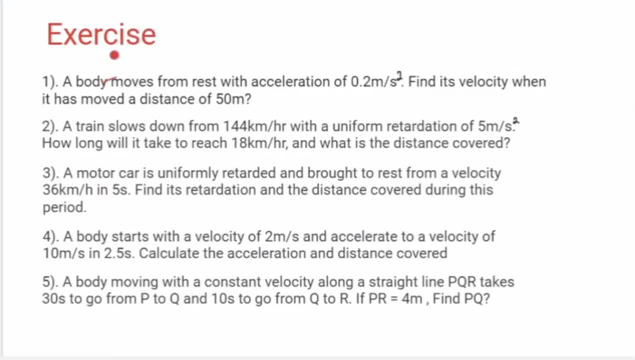 that becomes our answer: it is 7.5. all that becomes our answer: it is 7.5. all right, I would like you to do the right. I would like you to do the right. I would like you to do the following exercise: from question 1 to 5: 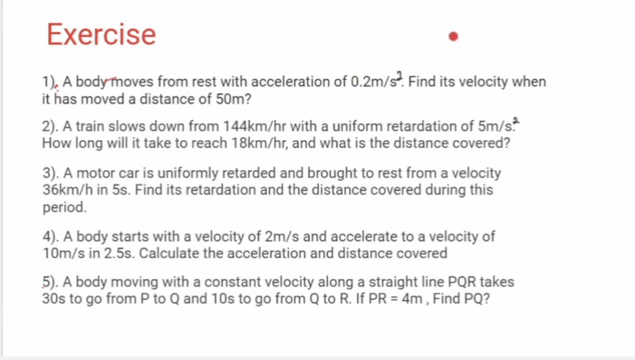 following exercise from question 1 to 5: following exercise from question 1 to 5: solve it. I like to get your feedback on solve it. I like to get your feedback on solve it. I like to get your feedback on how you deserve the question. thank you.